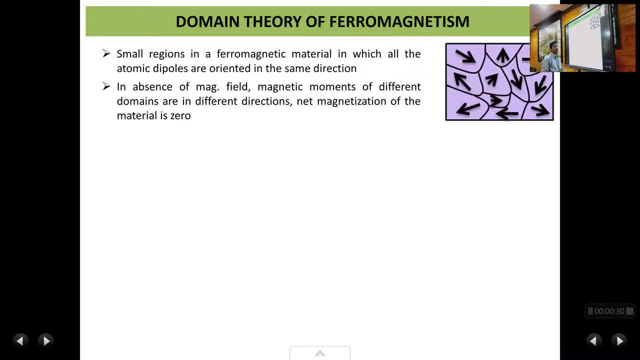 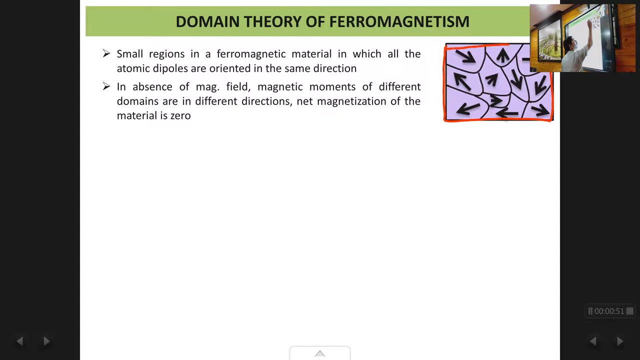 So what is the meaning of domains? So domains are basically small regions in a ferromagnetic material in which all the magnetic dipoles, all the atomic dipoles are oriented in one direction. So, for example, we have a ferromagnetic material over here In this material, so this is a ferromagnetic material. Now, this part over here is one domain. 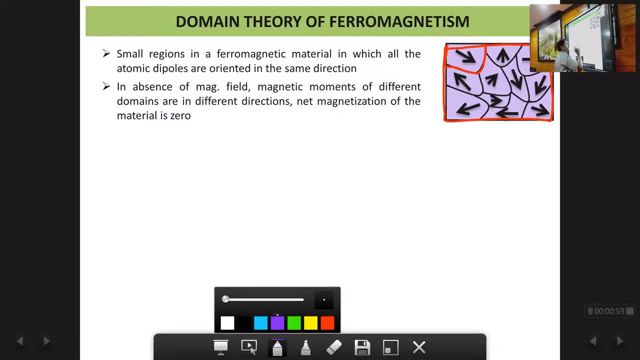 This is one domain. This is the domain of the ferromagnetic material. Now, what you see in that? so this is one domain, In that all the magnetic dipoles are oriented in this direction. So, if you sum them all up, the net magnetization is therefore in this direction. 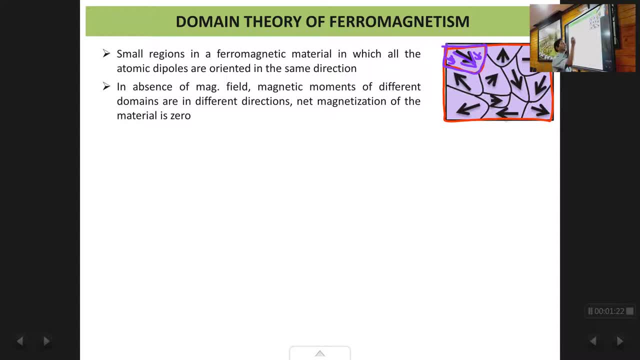 So this is in this region, this domain. If you consider another region, there another domain. so let us say this domain here, All the magnetic dipoles inside it are oriented in this direction, So that the net magnetization is therefore in this direction. 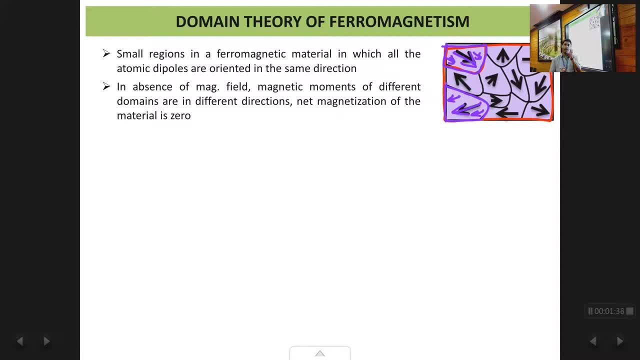 So, like that, the entire ferromagnetic material can be imagined to be made up of small, small regions in which all the magnetic dipoles in that particular one region are all pointing in the same direction. So this is called one domain. Different domains have different direction orientations. 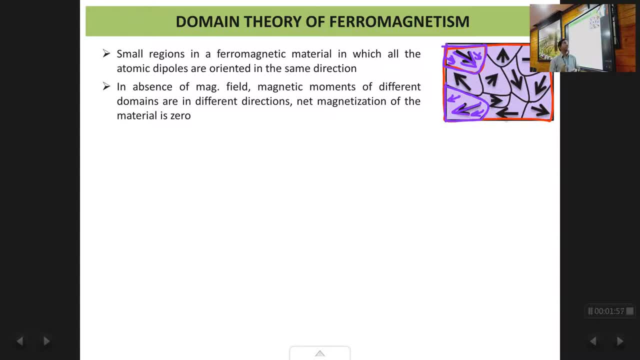 And that is why, in the absence of a magnetic field, the net magnetization is zero, because all the domains are randomly oriented. So if you sum the magnetic moments of all these different domains, the net magnetization comes to zero. So that is what we mentioned over here. 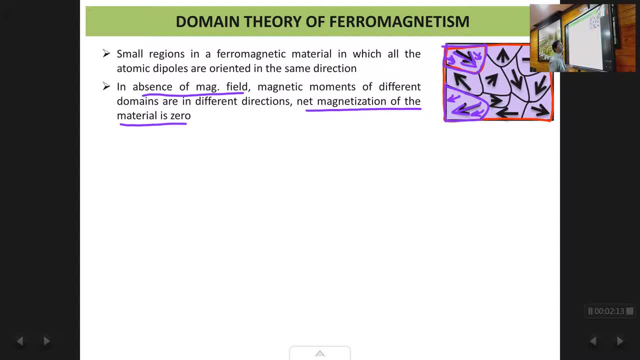 So, in the absence of a magnetic field, the net magnetization of the material is zero. But what happens when we apply a magnetic field? We know that a ferromagnetic material gets magnetized When we apply a magnetic field. So, with respect to these domains, what happens inside a ferromagnetic material when we apply a magnetic field? 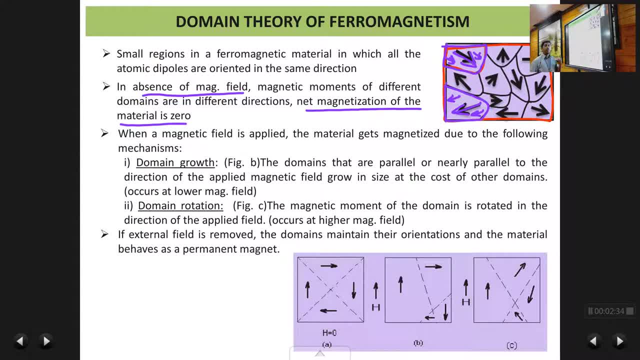 So there are two types of processes which take place inside the material when you apply a magnetic field. So what happens is so this first figure A here. what it shows you is the situation in the absence of a magnetic field. So the magnetic domains, individual magnetic domains, are randomly oriented. 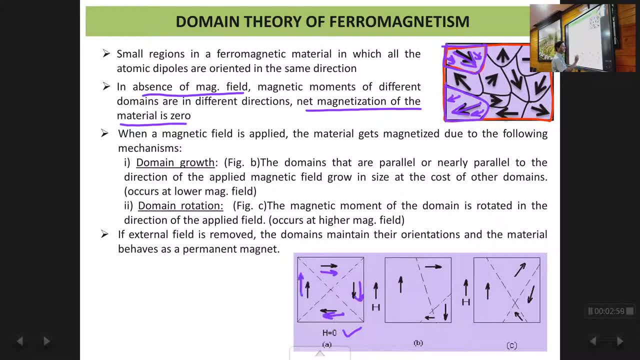 One this way, one down, one this way, one upwards, like this, So that if you see the sum of all these things, the net will come to zero. So net magnetization in the absence of a magnetic field is zero. Next, now, what we are doing is we are applying a magnetic field in this upward direction. 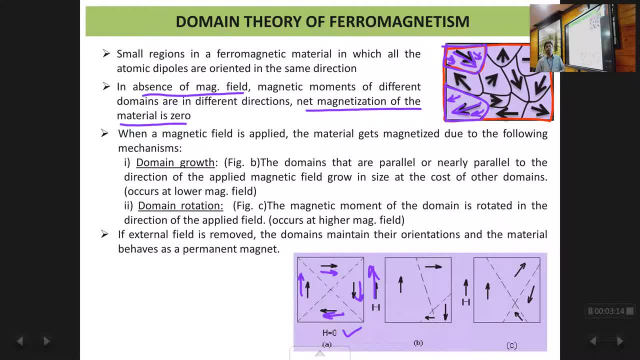 Magnetic field H, we are applying the material in the upward direction. So two processes take place over here which I have mentioned over here. One is called domain growth And the second one is called as domain rotation. Domain growth occurs when the field applied is less. 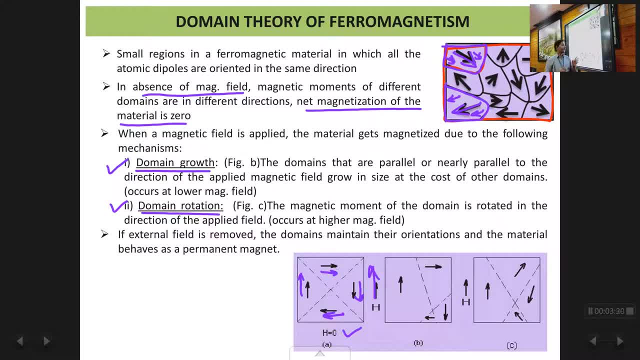 And as you keep on increasing the field, then the process of domain rotation starts occurring. So, initially, for low field values, domain growth process is more dominant, Whereas for higher field values the domain rotation process is more dominant. So what are these two processes? 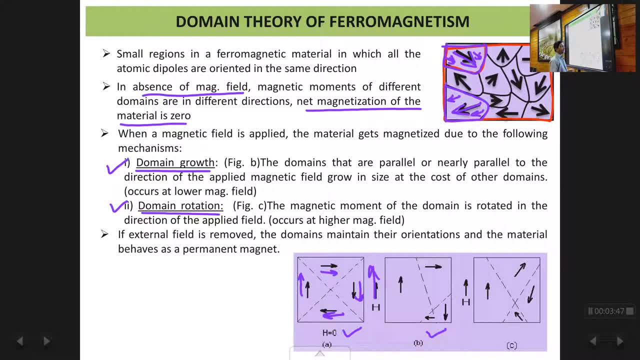 What happens in domain growth, which is shown over here in figure B. Since you have applied a field in this upward direction, whichever domain was in that direction of the field, the size of that domain increased. You can see this domain here, This domain, in the absence of magnetic field, it had a magnetic dipole, magnetic orientation in the upward direction. 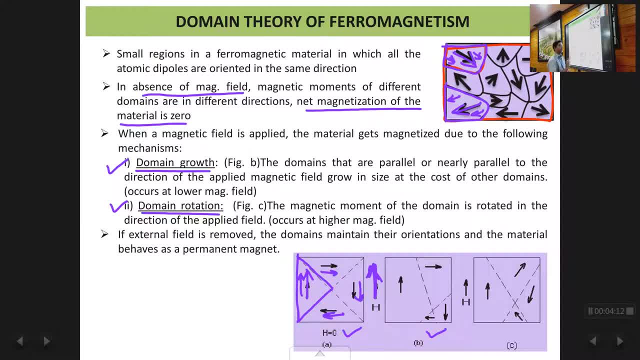 So, since the applied magnetic field is also in the upward direction, this domain here, this domain, it starts increasing in size at the expense of the other domains which are not in the direction of the applied field. So what has happened is this domain has increased, you see. 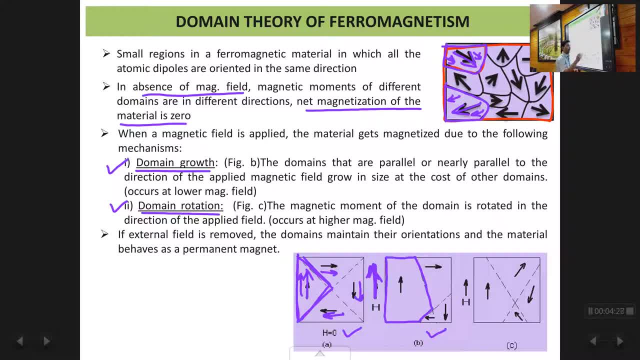 It has become bigger in size. And what has happened to the other domains? They have reduced in size. So the domain which is in the direction of the applied magnetic field increases and the other domains decrease. So this process is called as domain growth. 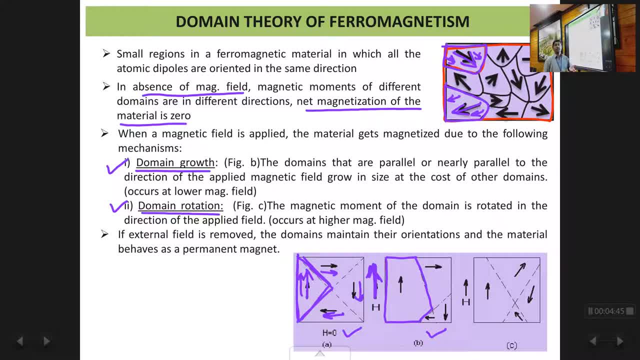 And this happens at low magnetic fields. But then, as you keep on increasing and increasing the magnetic field, there is a second process which also starts occurring that is called as domain rotation. So now what has happened is what has happened over here. this domain- initially it was in this direction. 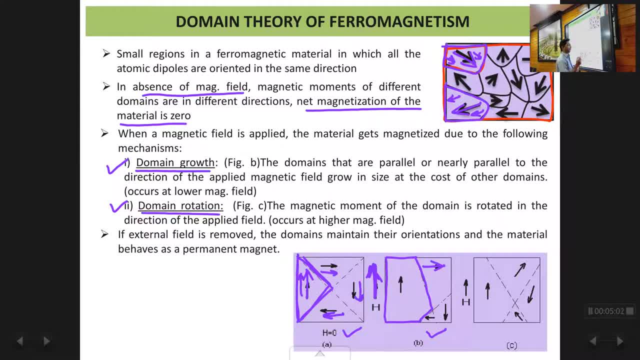 But now, as you kept on increasing the field, it also is trying to rotate upwards, Because the applied magnetic field is upwards. this domain was pointing towards the right, But now, since the field has become very large, high magnetic field is applied. 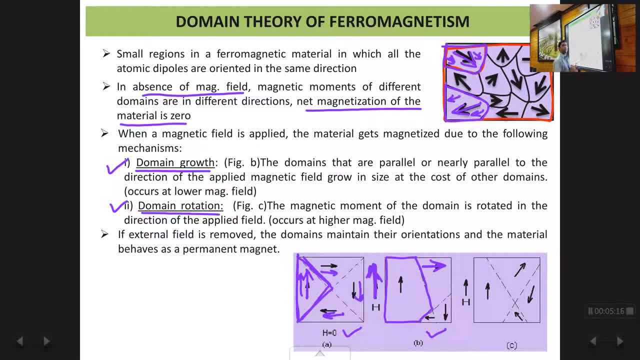 This domain also starts rotating in the upward direction. So you can see here. it has slightly rotated in the upward direction, This domain- over here it was pointing towards the left. It also has slightly rotated in the upward direction, as you can see over here. 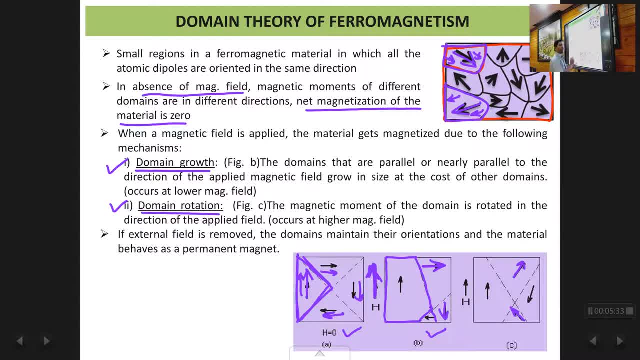 This domain also, which is completely down. it was completely in the opposite direction compared to the applied field. It was also slightly rotated and tried to come in the upward direction. So it was also slightly moved towards here the upward direction. So all the domains which are not in the direction of applied magnetic. 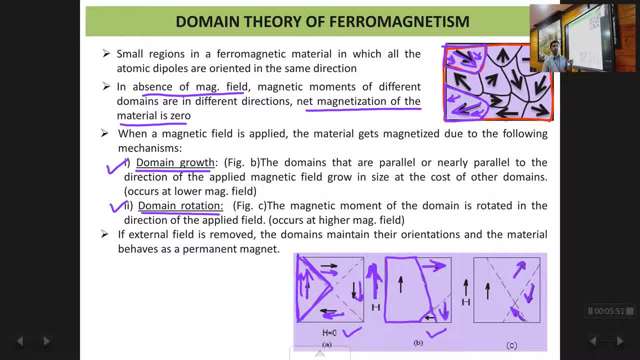 field. they rotate, the domains rotate, the magnetic moments in them rotate so that they are slightly pointing towards the direction of the applied magnetic field. So this process which is shown in figure C here, wherein the domains rotate, is called as domain rotation. The domain sizes remain the same, the full domain itself rotates in this process. So in the first process the 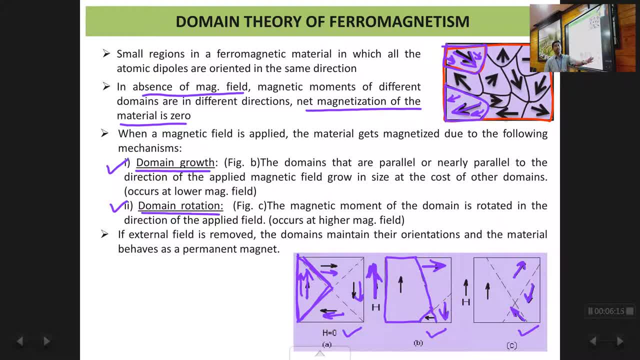 domain size increases in the favorable orientation, whereas in the second process the entire domains rotate in the direction of the applied magnetic field. So this is how the material gets magnetized. So now, if you see, in this figure A the net magnetization was zero. in figure B now the 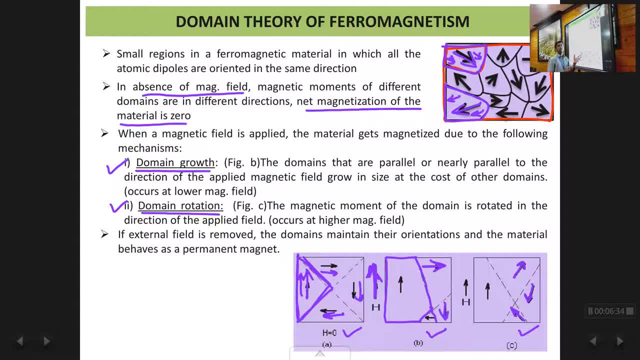 net magnetization will be upwards right because the major part of the material now has a domain which is in the direction of the applied field. So the magnetization is in the upward direction, so the material gets magnetized. Figure C: also the net magnetization. if you see the result of all that thing, it is in 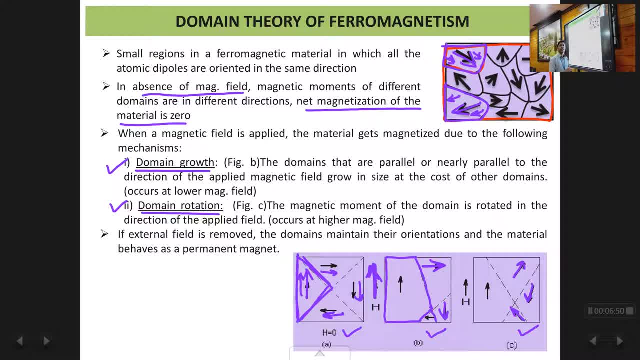 the upward direction. So this is how the material gets magnetized when you apply a magnetic field, and this is with respect to the domain theory. Now what happens is when your external field is removed. when you remove the magnetic field, these domains, slightly, may go back to. 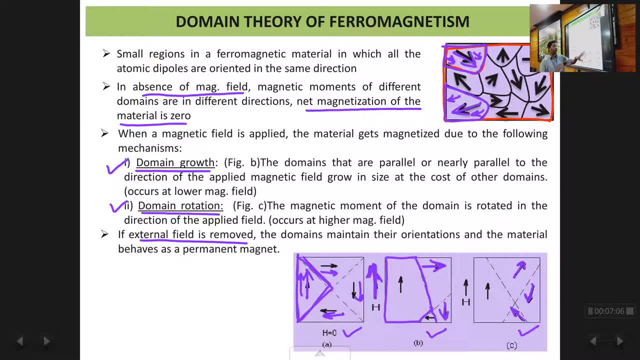 the original direction. they may also slightly reduce in size, but overall, whichever domains had increased in size, they almost remain the same size. they do not come back to the original size and original directions. So what happens is that the material still, even after removal of the magnetic field, it retains some of its magnetization. so and the material becomes. 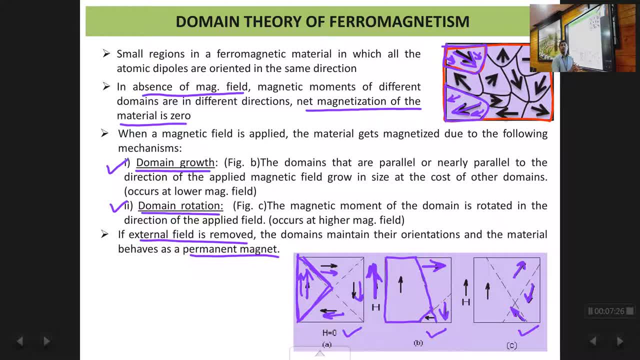 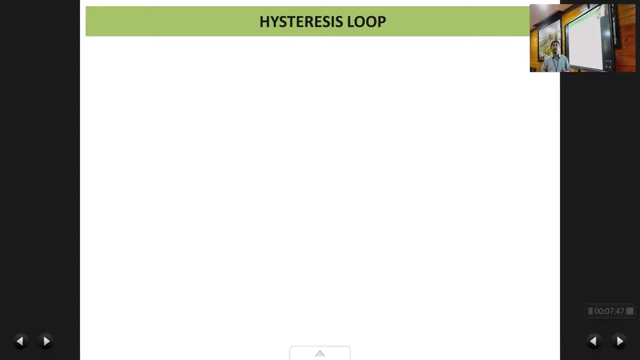 a permanent magnet. Why? because the domains do not come back to their original size or original directions even after the magnetic field is removed. So this is how we explain magnetization of a ferromagnetic material using the domain theory. The next important part in this chapter is also related to a ferromagnetic material is 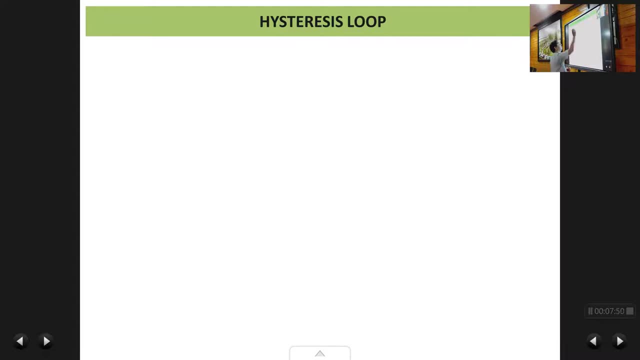 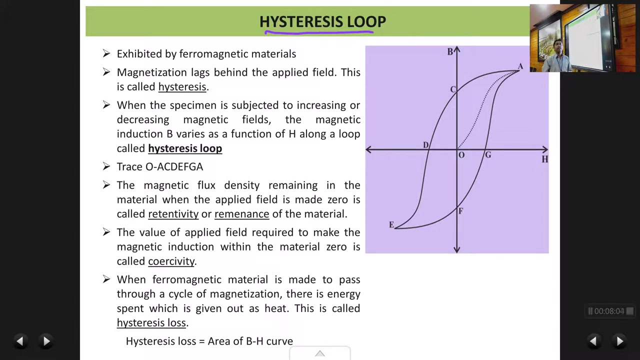 called as a hysteresis loop. So hysteresis and hysteresis loop, these are also properties only exhibited by ferromagnetic materials, not by a paramagnetic and diamagnetic. So what is this hysteresis loop? what is observed is that in a ferromagnetic material, the magnetization 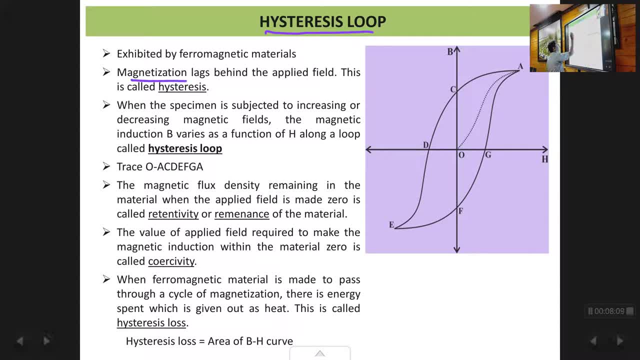 M, magnetization M lags behind the applied field H. Now the magnetization M, the magnetization M, the magnetization M lags behind the applied field H. So magnetization M lets behind the applied magnetic field H. So what it means by that: 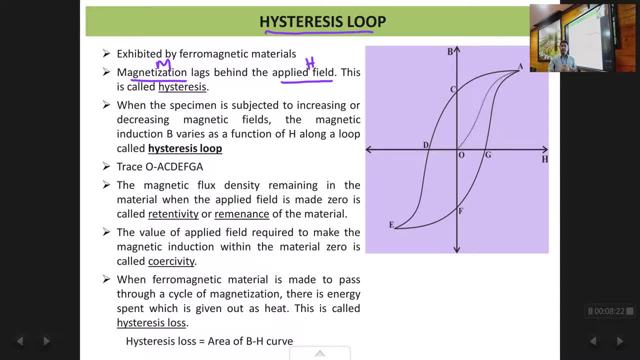 is that as you change the magnetic field, the magnetization also does not change in the same way as you change the applied field. So, for example, if you decrease the magnetic field by, let us say, 4 units, the magnetization also will not increase by the same amount- 4 units. 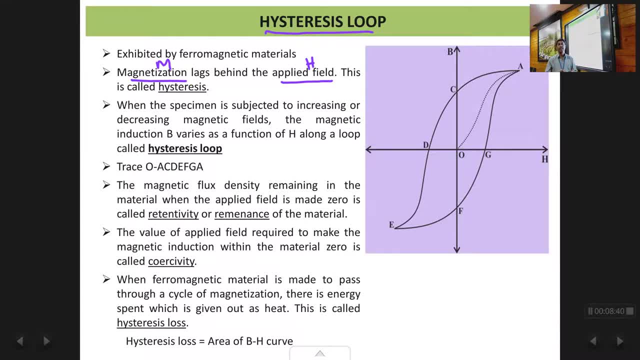 It may decrease by little, but not in the same extent as the decrease in the applied field. So you may change the field, but the magnetization will not follow the exact change in the applied field. So in other words, we can say that the magnetization is lagging behind the applied field. 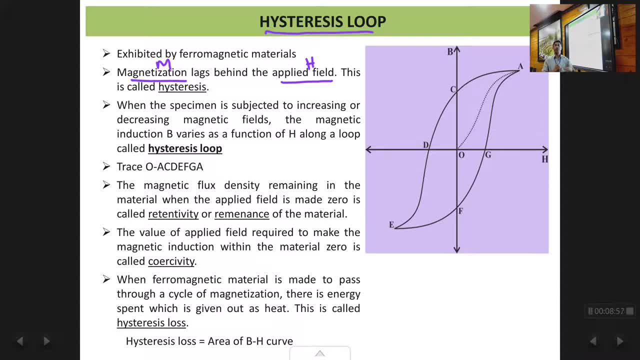 So you may change the field to a large extent, but the magnetization will not change to that same extent, So it is lagging behind the applied field. So because of this we get what is called as hysteresis. So hysteresis is basically difference. 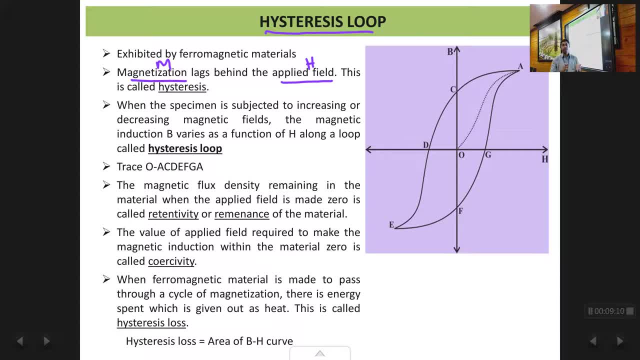 You are changing this, but the other thing is not changing to the same extent. There is some difference between the two things. So there is hysteresis between the magnetization and the applied magnetic field. So what is the hysteresis loop then? 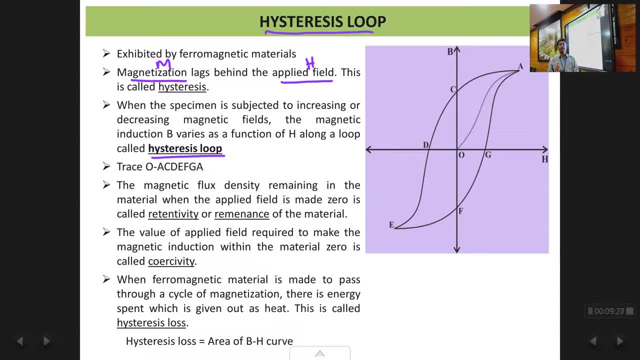 If we subject a ferromagnetic material to one complete cycle of magnetization, what is the meaning of one complete cycle? Let us say: you start from zero. You start from zero, You increase it, Make the field maximum, Then decrease the field. 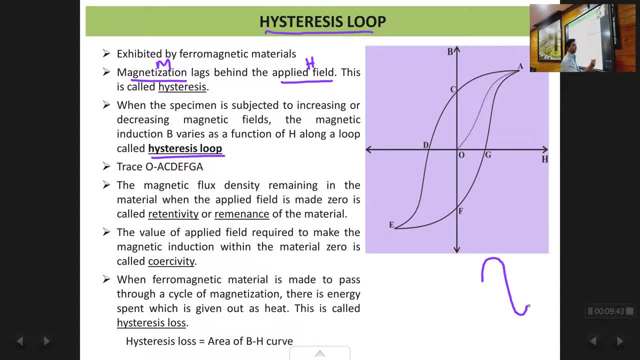 Come back to zero. Then you apply the field in the negative direction, Increase it in the negative direction and then come back to zero. So this is one cycle. It is like an AC signal, So one full when you run the magnetic field into the ferromagnetic material over one complete. 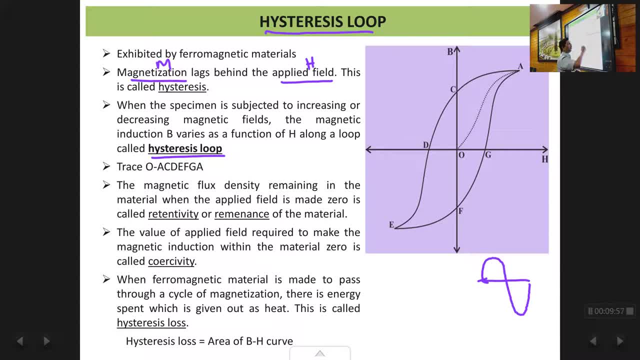 cycle, we get such type of a loop formation which is shown in the figure here, And this is called as a hysteresis loop. So basically, hysteresis loop arises because the MH3. So this is called as a hysteresis loop. 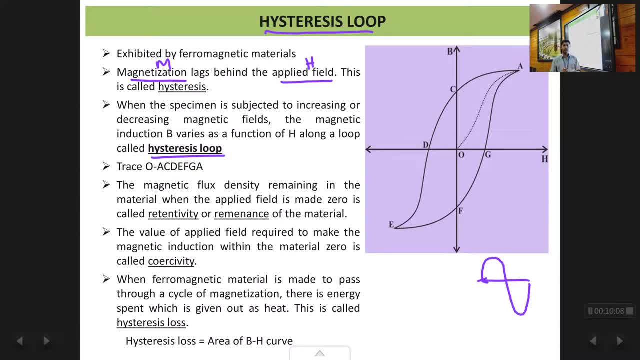 So basically, hysteresis loop arises because the MH3. So this is called as a hysteresis loop. This is sensitive present if used. So that is the syntactic loop. There is some magnetic fields and the magnetic field in the magnetic field is y. 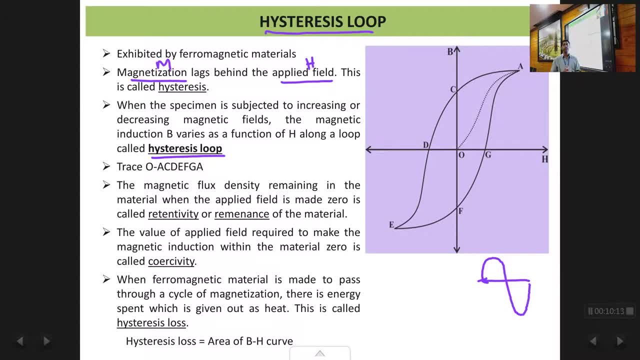 So this is Exactly Y üç���습 game, because of what we have labelled of it Is the H Magnetization. 0 is 0.. 0, 0. all right, it is zero and we start with a zero magnetic field also. so it is zero comma, zero magnetization. 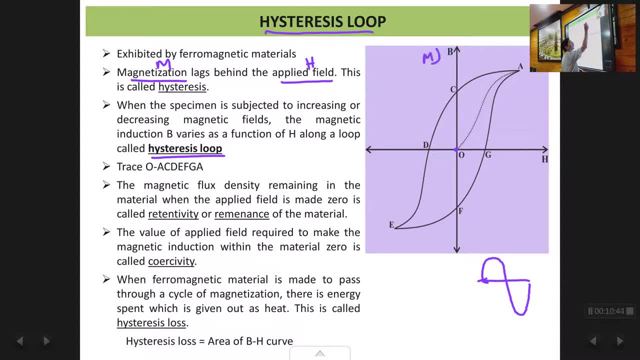 also is zero and, by the way, this b, we can also replace it with m. okay, so because remember formula for b and m: magnetic induction b and magnetization m. they are related, as b is equal to h plus m, so as as you increase magnetization, automatically magnetic induction b also increases. 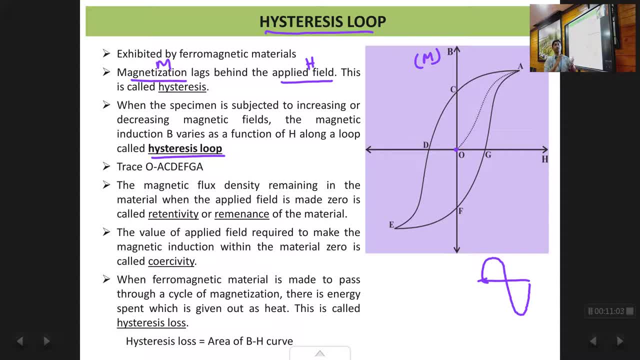 okay, so as m increases, b also increases, so we can always interchange between b and m. okay, so magnetization of magnetic induction is along the y axis and applied magnetic field is along applied magnetic field. h is along the x axis. so now to start with. we started. 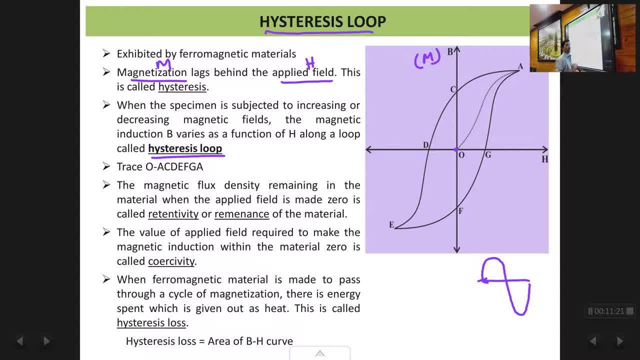 the armagnetized sample and we started with zero magnetic field. so it is zero comma zero at point o. then as we increase the magnetic field, the magnetization also increase. you can see this graph: there is the increase as the magnetization also is increasing. and then 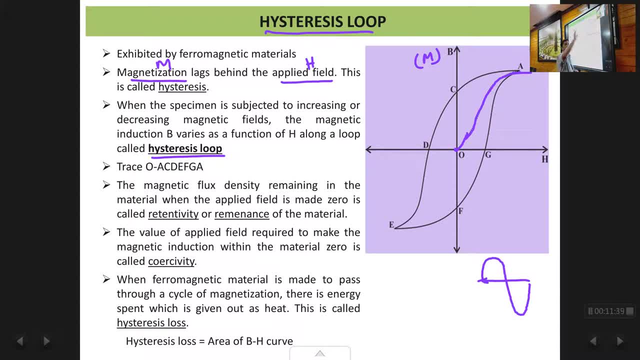 it switching of both magnetic field. so here, because from point o we can multiply, it even starts to become constant, starts to become saturated value. ok, towards point a. if you keep on increasing it it will attain a constant value that is called as saturation. so that occurs at point a. let us say so beyond point a. if you increase it, the magnetization will. 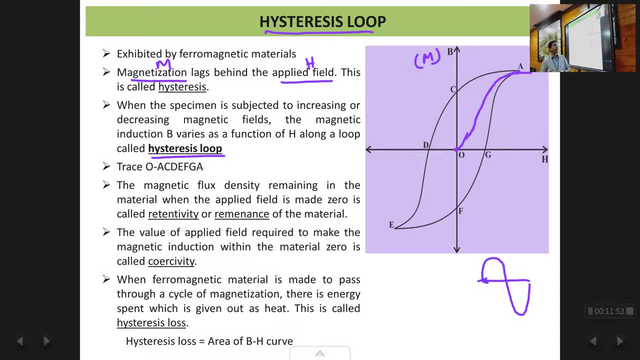 remain the same value as indicated at point a. so what has happened? initially, as we increase the magnetic field from point o, the magnetization also has increased, and then it has attained the constant value next. yeah, so from o to a, as we increase the magnetic field, the magnetization 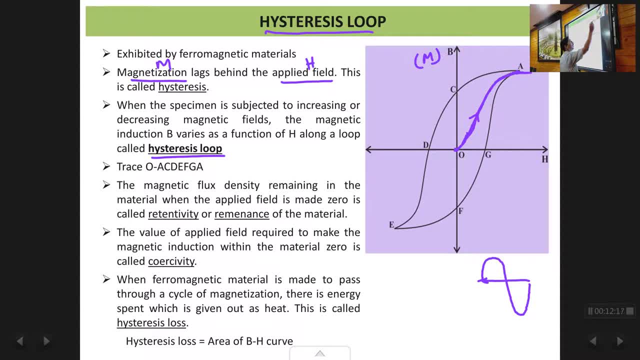 also is increasing. it reaches saturation at point a. then, as we now decrease the magnetic field, as we are coming back towards zero, so we are decreasing the magnetic field. you see, the magnetization does not trace the same path it had traced from o to a, it rather goes. 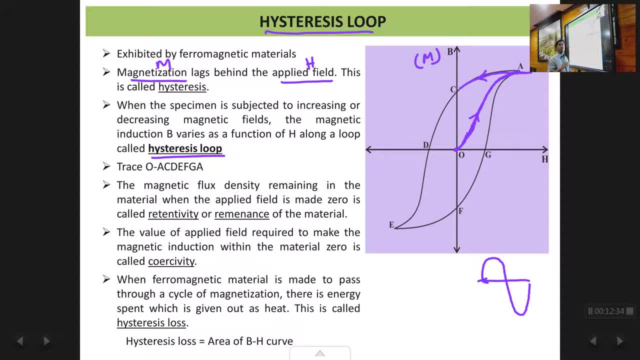 from along another direction, another path, ac. so what we see over there is that whatever path initially the magnetization had taken while reducing the magnetic field, it does not come back on the same path, it follows a different path. and what is important to note is that at point c, the value of magnetic 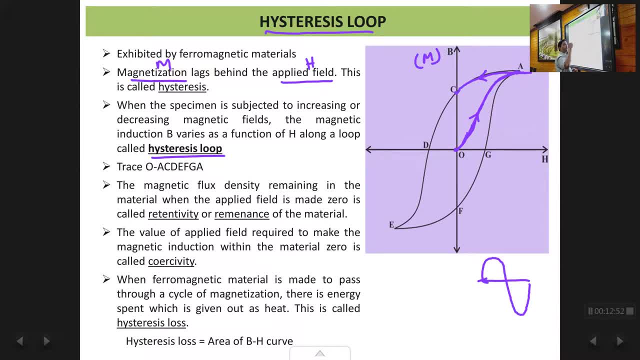 field h is zero because it is at along the y axis. so h value is zero, but the magnetization m is still not zero. so this much value is still remaining. so this value, oc, is zero. this is what is still the amount of magnetization remaining in the material, and this oc is called. 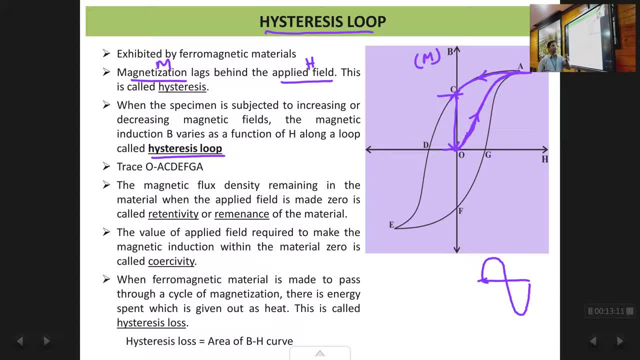 as the retentivity or remanence of the material. so this oc value tells us how much amount of magnetization still remain in the material even after you remove the magnetizing field h. ok, so that's what we can see over here. the magnetization is lagging behind the applied. 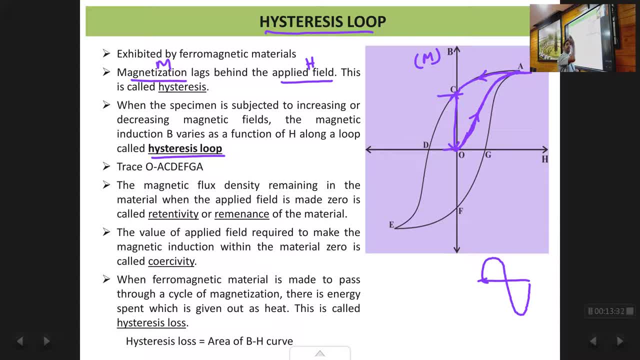 magnetic field. we have made the magnetic field zero but the magnetization still not become zero. so magnetization is behind the applied field, so it lags behind the applied magnetic field. then as we further decrease the magnetic field, further decrease it in the negative direction. 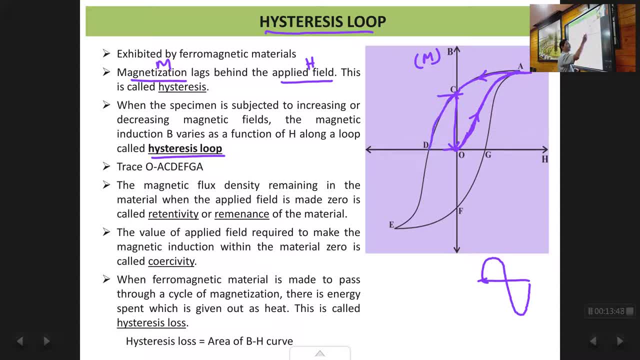 the magnetization from point c it is decreasing. coming to point d, at point b the magnetization becomes zero because you can see it is on the x axis. x axis means m value or b value is zero. so at point d the magnetization becomes zero. 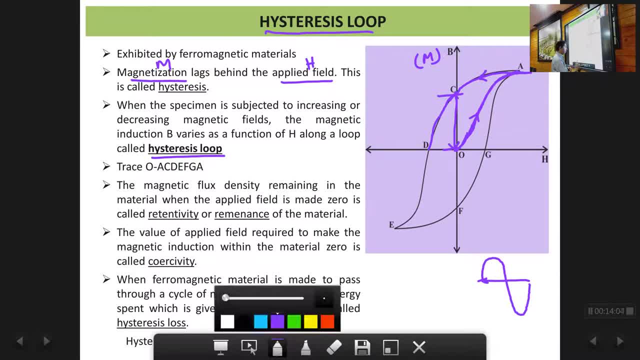 so this amount of magnetic field which you require, the amount of magnetic field required to make the, this value from here to here, the amount of magnetic field required in the reverse direction to make the magnetization in the material zero, is called as the coercivity shown over here. so retentivity is the magnetization retain the material even upto the magnetic 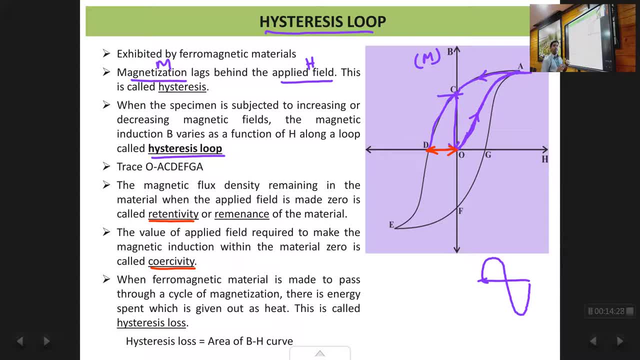 field is made zero. that's the retentivity, where as coercivity is the magnetic field required to make the magnetization in the material zero. so then, as we continue further, if we further decrease the magnetic field in the negative direction, the magnetization starts increasing in the negative direction. it again attains the saturation value: negative saturation. 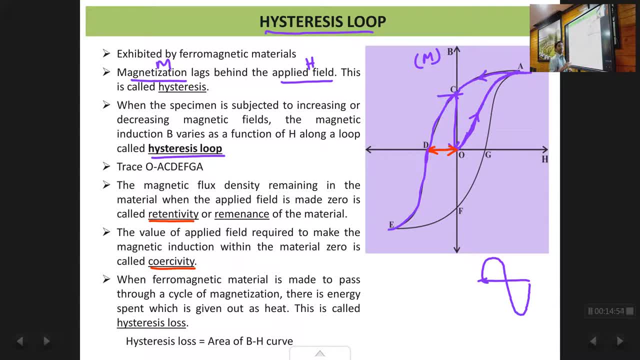 value at point e. if you continue to decrease the magnetic field further in the negative direction, the magnetization will no longer further increase. it retains the saturation value. then if we start again increasing the magnetic field towards the positive direction, towards 0, then in the magnetization follows this curve EF again at F the field has become 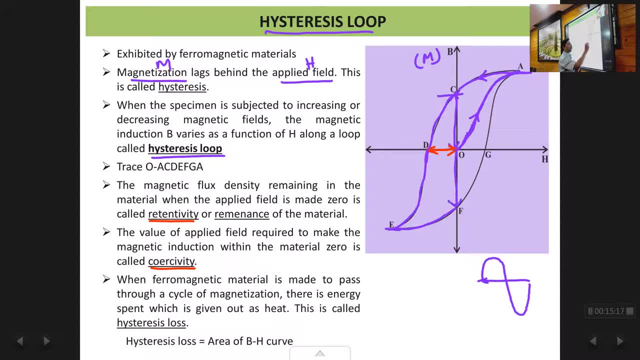 0, but the magnetization is still not become 0. so this again is the retentivity. so retentivity is either OC or OF. both are exactly equal. it is a symmetrical curve. so OC and OF, both are what can be called as the retentivity. 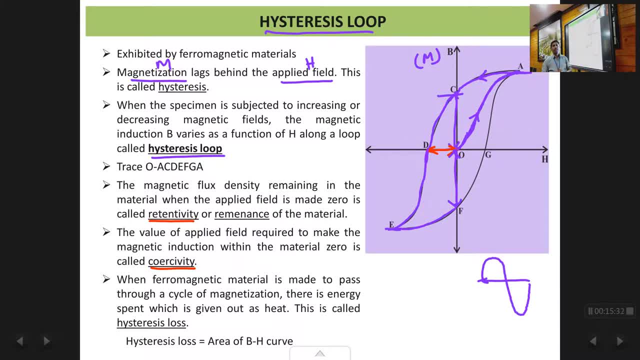 OC is retentivity in the positive direction, OF is the retentivity in the negative direction, but in value they both the same. then if you again start increasing the magnetic field towards the positive point, again the magnetization increases. from F to G the magnetization decreases. 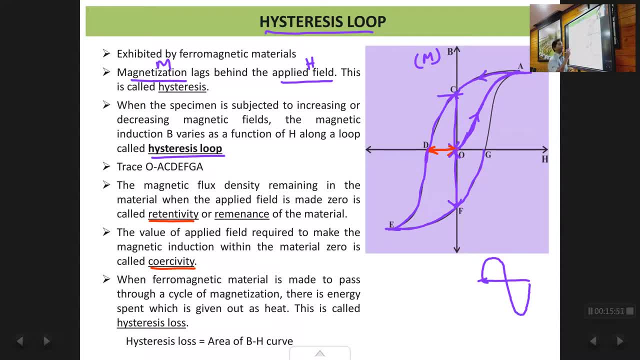 sorry. And at the point G it is fine, it becomes 0 again. so this value again, OG is also the cohesivity. so this value, OG is also the cohesivity, but in the positive direction. so OD and OG, both can be said to be as cohesivity. 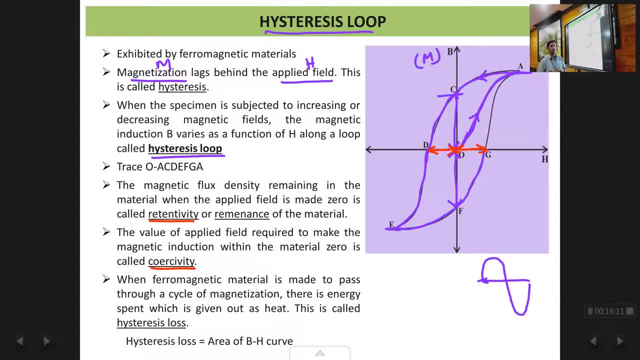 the values are same but they are in opposite directions. one is positive, one is negative, and then further you increase the magnetic field from G. if you further increase it, it goes along this path, GA, and then it continues. so this cycle you started from 0. you started. 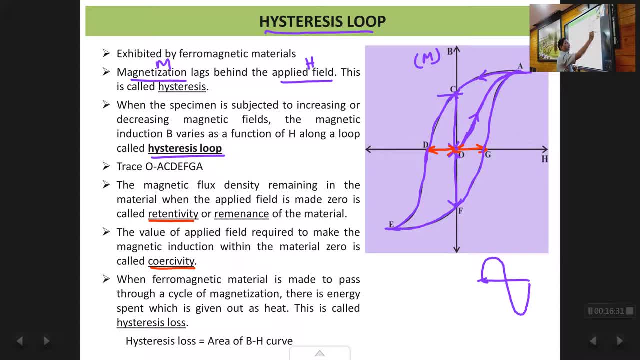 from 0 you went: increase the magnetic field towards a large value, then you came back towards 0, then increase the magnetic field towards a negative direction, then you came back to 0 and then you continue the cycle. so this is like one full cycle: positive, negative, 0. 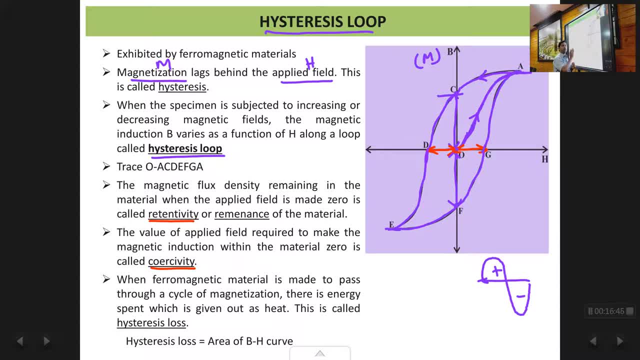 to positive, to 0.. So this one full cycle of the applied magnetic field and the hysteresis loop is traced in this way: as you vary the magnetic field for one full cycle, positive and negative. and now remember this curve: OA will never be traced again. it is only in the beginning trace OA. 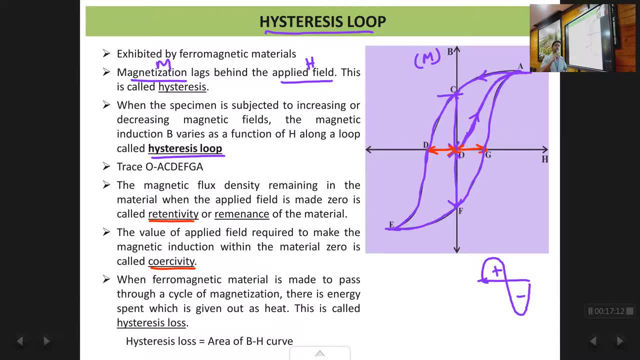 you will get it only when you start with the unmagnetized sample. once one full cycle of magnetization is run over the sample, the curve OA will never be traced again. it will always go along A, C, D, E, F, G, A, and then over and over again along the same direction. so 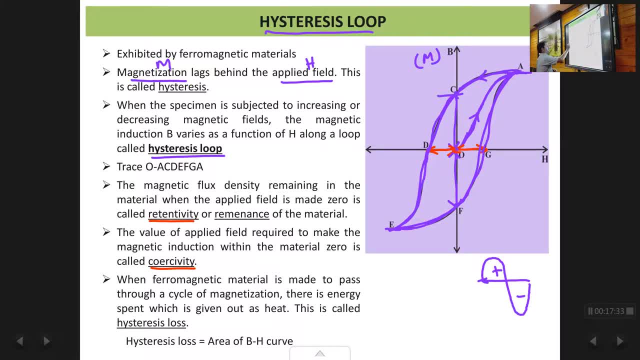 that is what is the hysteresis loop here, see. so O initially, to start with the unmagnetized sample. you start from O, then from O it goes to A, C, D, E, F, G, A and then it runs over the same direction. So this is the hysteresis loop. 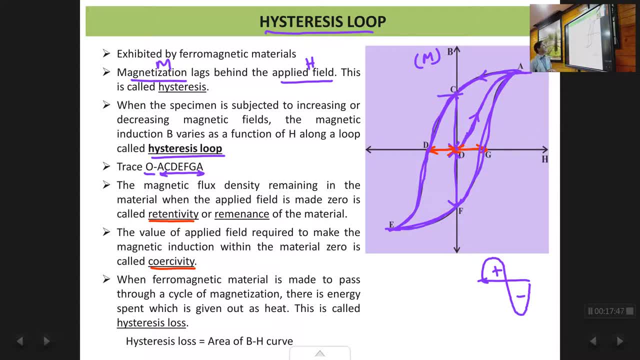 It repeats over and over again along the same thing: A, C, D, E, F, G, A, and this is nothing but the hysteresis loop. So we have already defined what is retentivity and cohesivity. these are two important definitions which you need to know. 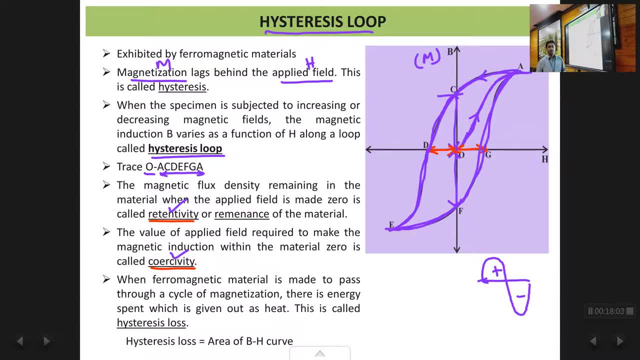 Now, last thing regarding the hysteresis is what is called as hysteresis loss. Now, when you run the magnetic field for one full cycle, there is a heat generated in the heat which is generated in the ferromagnetic material. So, for example, if you touch a transformer or any other motor of A C motor, you will feel. 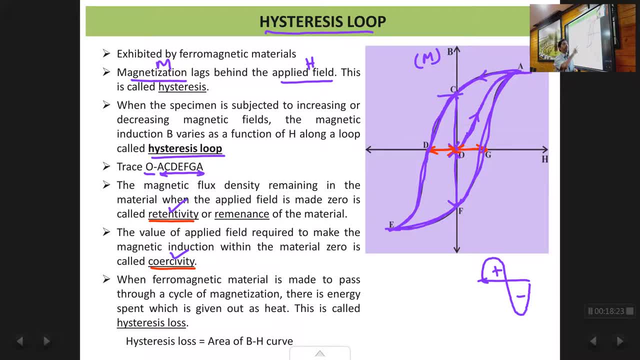 the heat in it. Why? Where does the heat come from? It is basically the amount of heat loss. for the magnetization to increase, come back to zero, increase in the negative direction and then come back to zero. For one running of one hysteresis cycle, the energy which is lost in the material is coming. 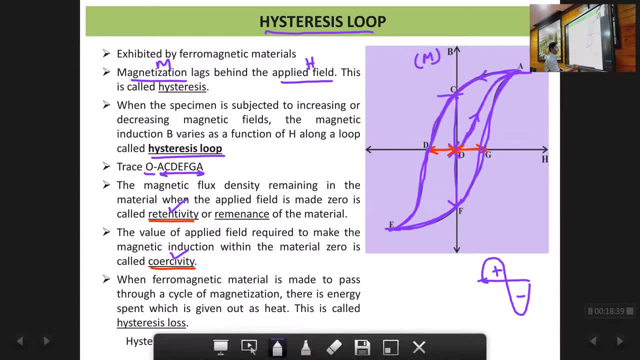 out as heat. So what is the hysteresis loss? Hysteresis loss is nothing but the area under the loop. Whatever is the area under the loop, the energy which is lost in the material is coming out as heat. So what is the hysteresis loss? 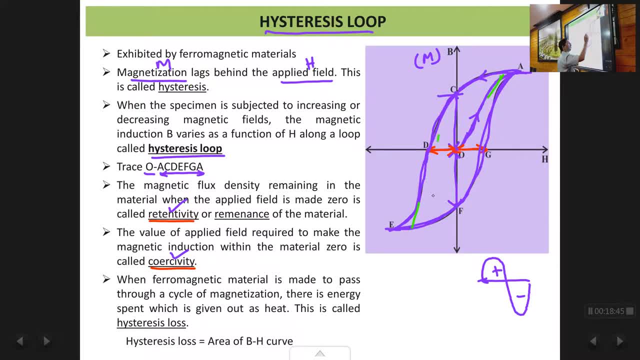 Whatever is the area under the hysteresis curve, this area gives you the hysteresis loss, the amount of energy lost in one full cycle of the magnetization. So hysteresis loss is equal to area of the B H curve or area of the M H curve. 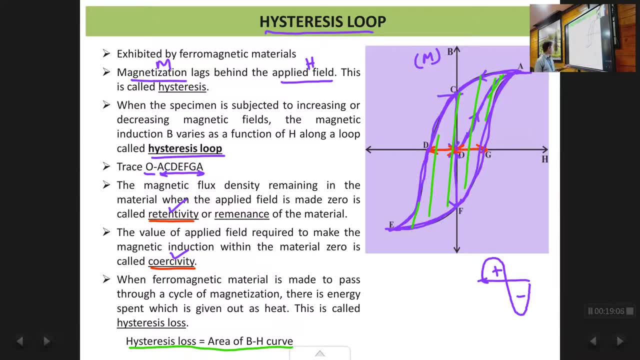 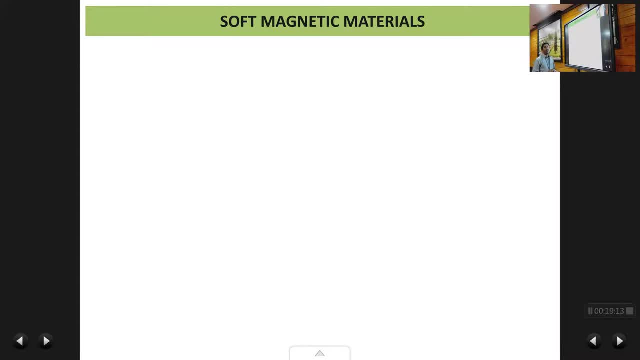 Area of the hysteresis loop gives you the hysteresis loss in one cycle of the A- C magnetic field. Now ferromagnetic materials are classified into two categories: soft magnetic materials and hard magnetic materials, And this classification is done based on the type of hysteresis loop which they generate. 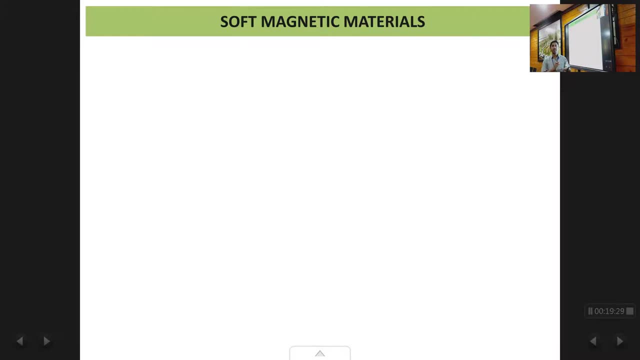 You subject them to a A C magnetic field for one full cycle, The hysteresis loop which they produce. based on that, we classify them either into soft magnetic materials or hard magnetic materials. So what are soft magnetic materials? Those are, They are: 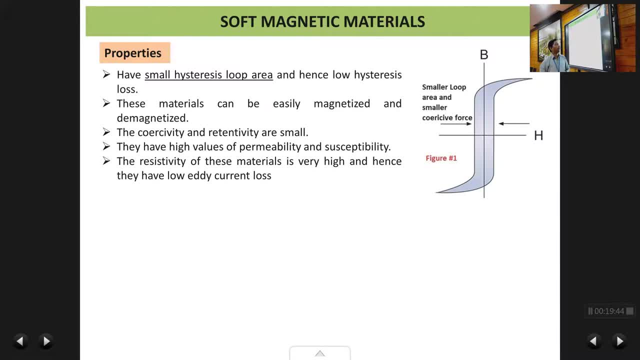 These are the materials which form a very small hysteresis loop. So you see, the area of the hysteresis loop is very small over here. for a soft magnetic material, The cohesivity value which you see here and here is also very small. 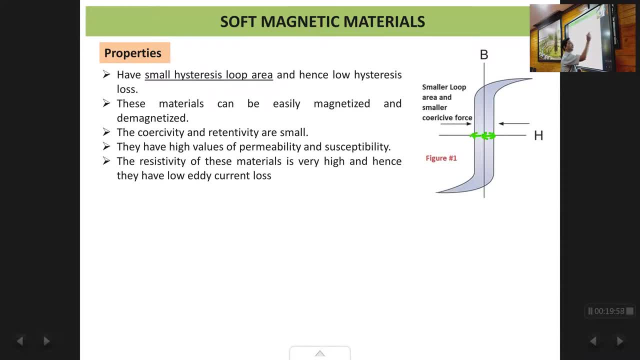 This is the cohesivity, or this is the cohesivity. They are very small values. So what does it mean? is that these materials soft magnetic materials? it is very easy to magnetize them and very easy to demagnetize them also, So do not require a very small amount of magnetization. 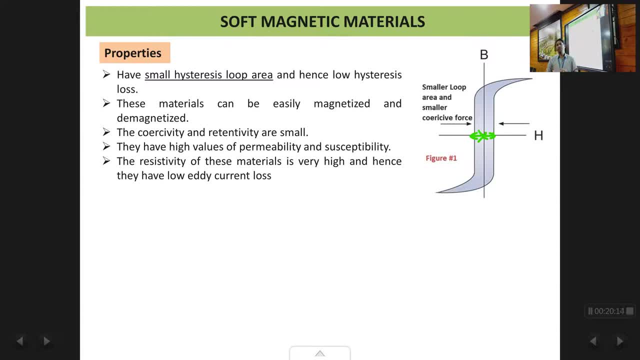 Do not require a very large magnetic field to demagnetize them. Very small magnetic field is enough to demagnetize them. So that is why they are called as soft. They can easily be magnetized and demagnetize. So we have a small hysteresis loop. 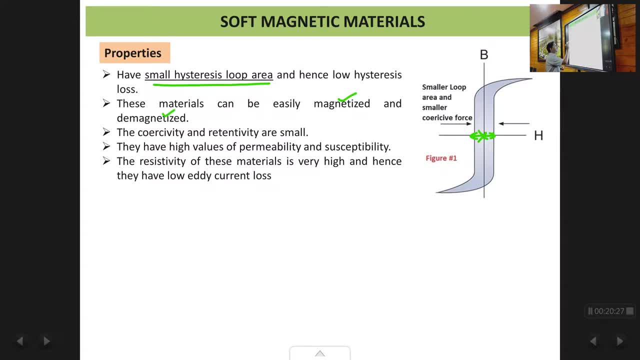 These. They can be easily magnetized and demagnetized. The cohesivity and the attentivity are small. As I already mentioned, cohesivity and the attentivity of the materials are also very small, So because of that, these materials are mostly used for. 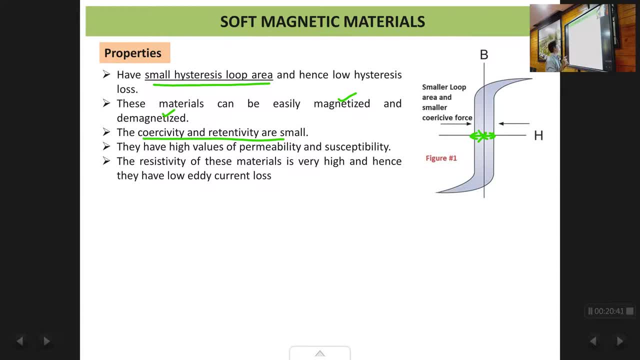 For To magnetize. we will come to the application later on. probability and susceptibility of these materials are high, so mu value and high value of soft magnetic materials are high. resistivity of these materials is also very high, so therefore the eddy current losses so current if the resistance of the 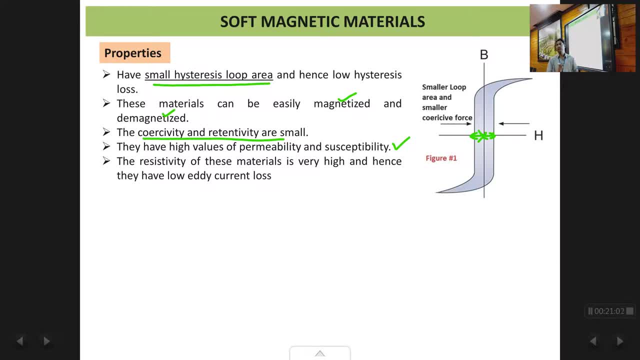 material was less, current would have been more and eddy current losses would have been more. but this soft magnetic materials have a high resistivity, hence the eddy currents in it are less and so the eddy current losses also in it are less. so these materials, where 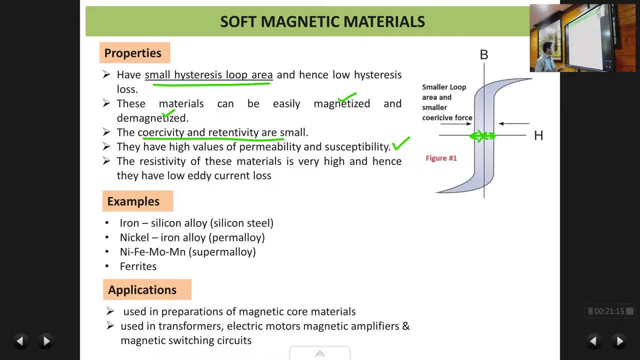 are they therefore used? they are mostly used to make cores in transformers in motors because, you remember, if too much of heat services loss is there, too much of energy will be wasted in the transformer core, on the core of a electric motor. so soft magnetic materials which can 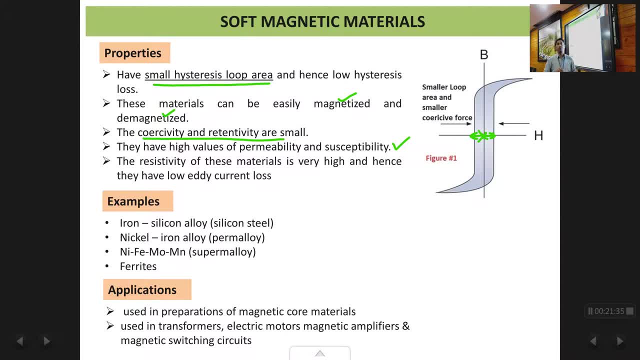 be easily magnetized and demagnetized, are therefore used in soft ion cores of transformers and magnets. So these are some of the soft magnetic materials which are used in transformers, in other machines which require a magnetic core inside them. Example of soft magnetic materials are: ion- silicon alloy- nickel ion alloy- nickel ion. 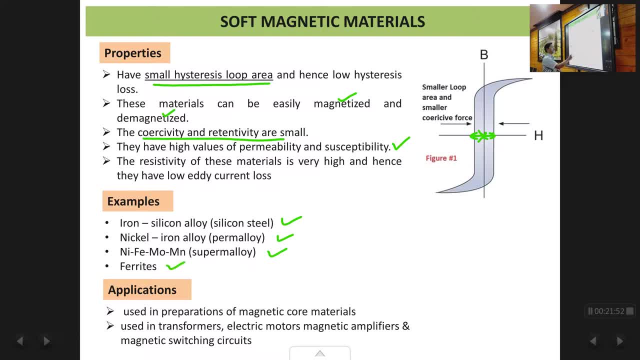 molybdenum and manganese alloy and all the ferrites. there are certain classes of materials called ferrites. all these ferrites are soft magnetic materials. so these are the ferrites which are only used in transformer cores because they have a very less heat service loss in. 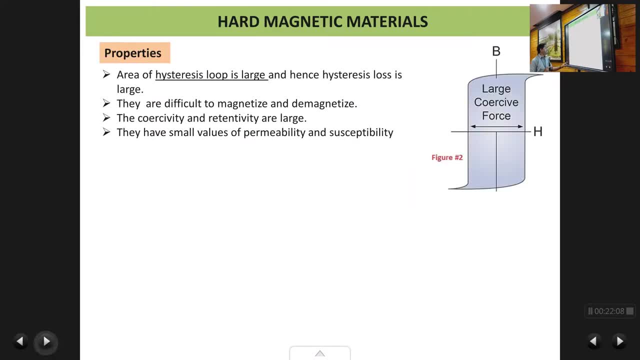 them. Now, materials are hard magnetic materials. you can see the area of heade resist loop over here is large. ok, so the coexisting ratio is quite the large value for hard magnetic material. so it is difficult to manganetize if you start the process to do so. it is difficult to de magnetize it. you will require to apply a very 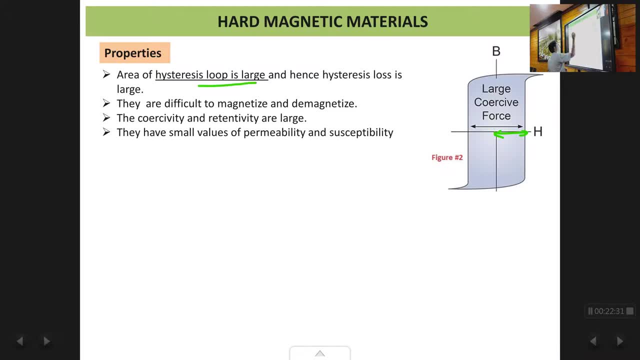 large magnetic field in a reverse direction to de magnetized this materials. so they have a large heade resist matrix area and it is difficult to de magnetized them and they have high value of cohesivity and retentivity. probability and susceptibility values are less. 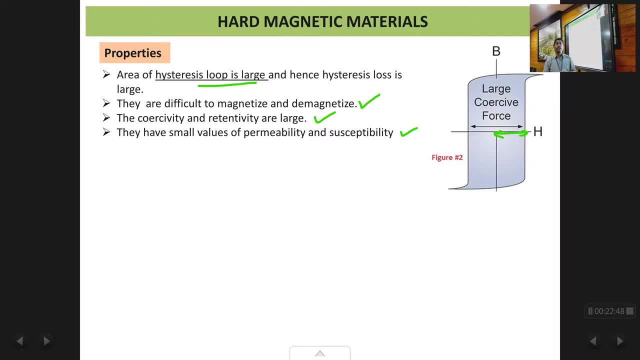 so mu value and chi value for hard magnetic materials are small values. so where are the examples of hard magnetic materials? are carbon, steel, tungsten, chromium, steel and alnico. its, an alloy of aluminium, nickel and cobalt. its the most commonly used hard magnetic material, alnico. 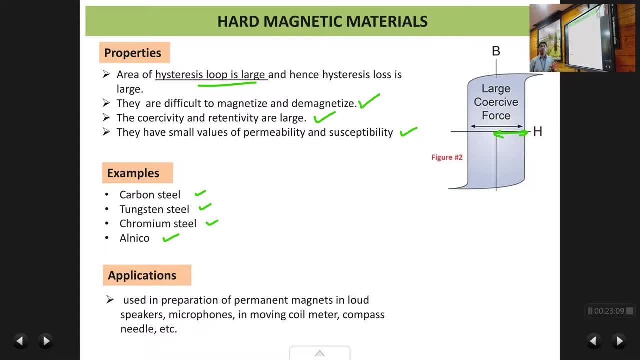 and applications. they are used wherever you require a permanent magnet, so hard magnetic materials are mostly used to make permanent magnets. so where do you find permanent magnets? you find them in dc motors. you will find them in loud speakers, then in your compass. ok, the magnetic needle of a compass- north, south pointing compass- is actually a permanent magnet there. 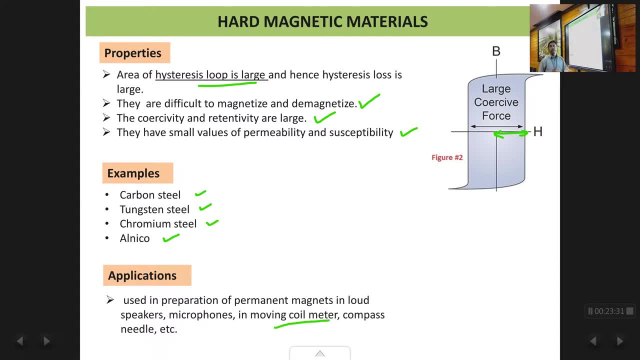 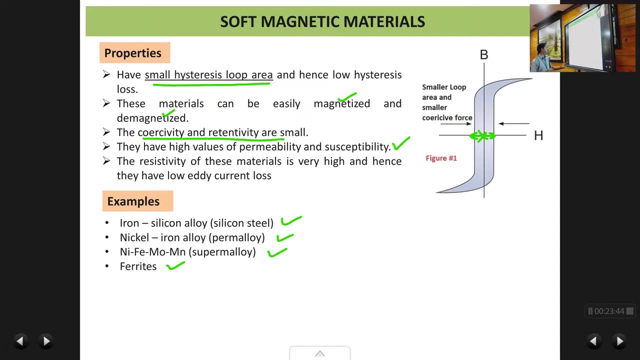 then the moving coil nanometers, moving coil voltmeters, ammeters, ammeters. they have a permanent magnet in them, so any device which requires a permanent magnet, use hard magnetic materials over there. so these are the types of soft magnetic materials and hard magnetic materials. 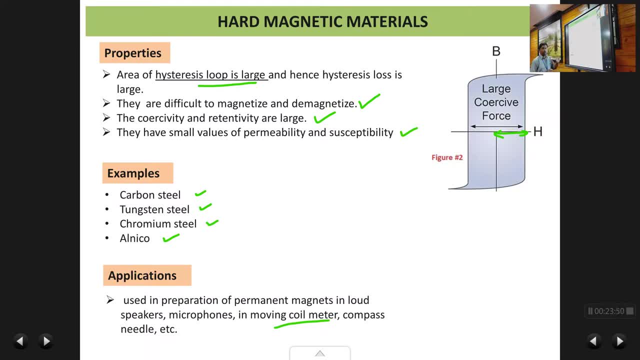 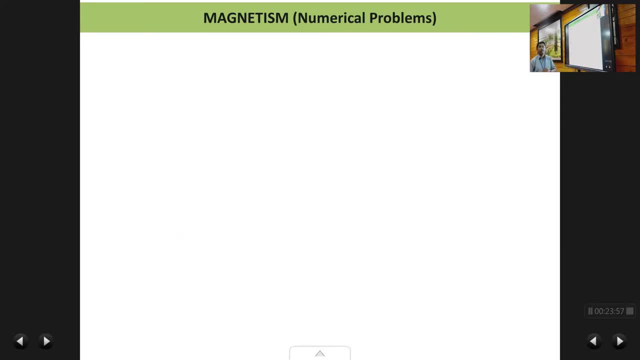 remember, both of them are ferromagnetic in nature, so ferromagnetic materials are either hard or soft. so with this we come to an end of this chapter on magnetism. there is another first part of the magnetism chapter. there is another part of CRO, which I will do in a next class. 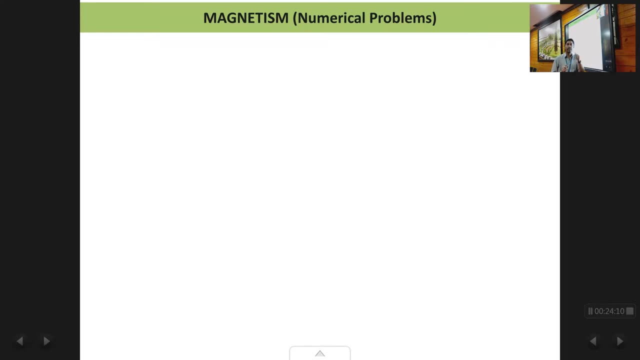 rather CRO is a slightly big topic. but CRO, remember it, comes under in the same chapter of magnetism. so we will do that in a separate class. but before we end this class I will do just one example: numerical problem in this chapter of magnetism. 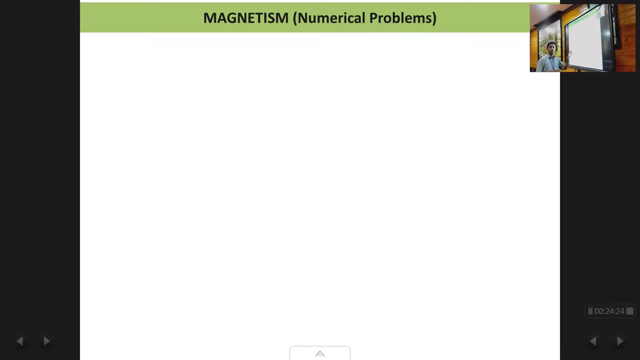 ok, so there are very few problems in this very small chapter, first of all on magnetism, and there is basically one or two problems which have come in the question paper based on this chapter. so we have a problem over here. a magnetic material with susceptibility of 0.3 x 10 raised to the power minus 5. 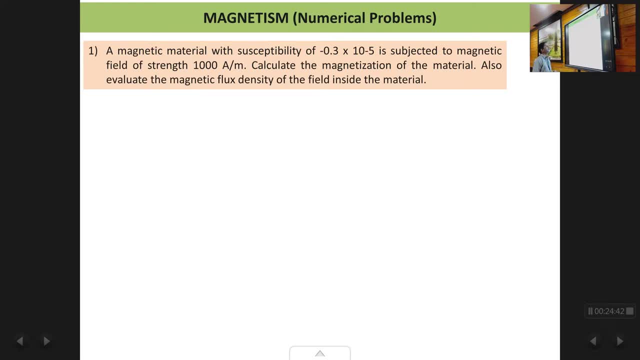 is subjected to a magnetic field strength of 1000 ampere per meter, calculate the magnetization of the material and also calculate the magnetic flux density of the field inside the material. so what is given to us over here is magnetic susceptibility, that is, chi. chi is given to us as magnetic flux density. 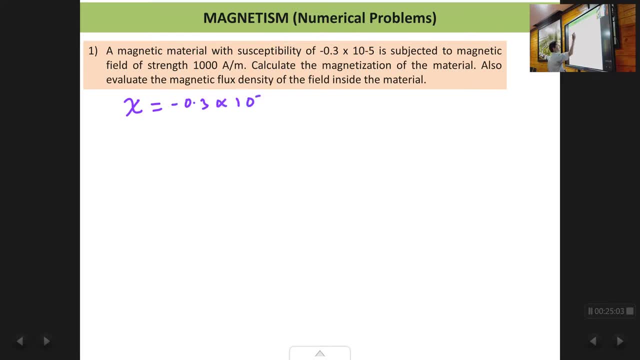 minus 0.3 x 10, raised to the power minus 5. remember, chi does not have units, it is a dimensionless quantity, so no units. what else is given to us is magnetic field strength. so H is given to us. H is given to us as 1000 ampere per meter. 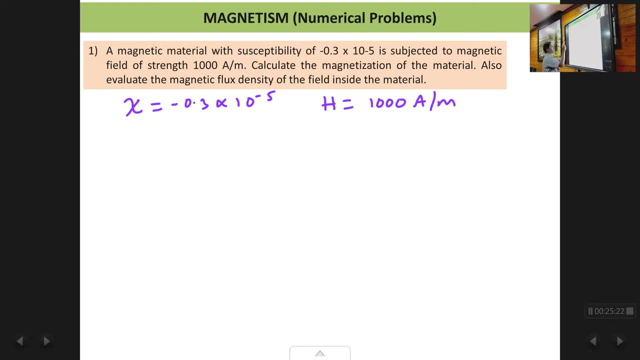 we are required to find what is the magnetization? so what is M? we need to find this and also we need to find magnetic flux density, which is B. so two things we need to find in this problem: one is the magnetization and one is the magnetic flux density, or magnetic induction. 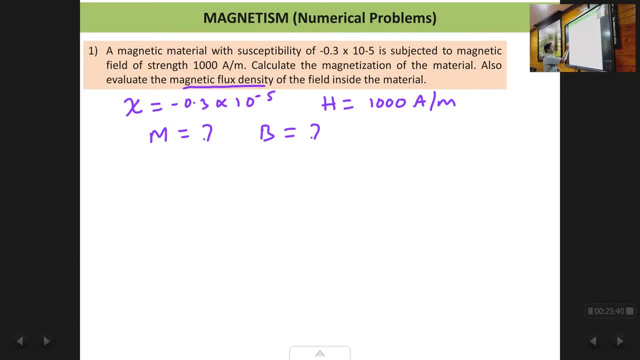 so how to find M? it is very simple to find the value of M. remember the relation which M and magnetization and applied magnetic field. so magnetization is chi times H. remember we had said that magnetization is directly proportional to the applied magnetic field H, and the proportionality constant in them is chi. 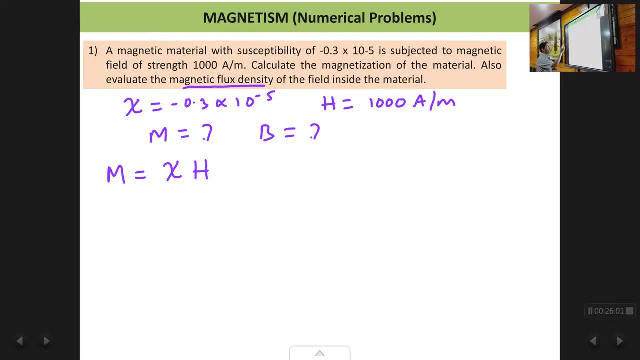 so M is equal to chi times H. so you just think that as we find the value of magnetization, so this is minus 0.3 x 10 raised to the power, minus 5 into 1000, so this value will count to be. so this is minus 5 and this is 10 raised to 3. 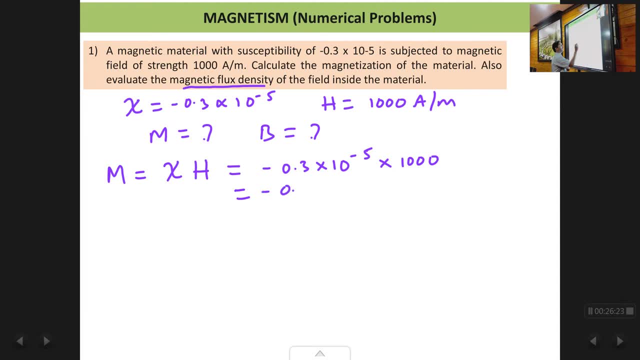 1000 means 10 raised to 3, so it will become minus 0.3 x 10 raised to the power, minus 2. and what are the units of magnetization? magnetization will have the same units of applied magnetic field, which is H. 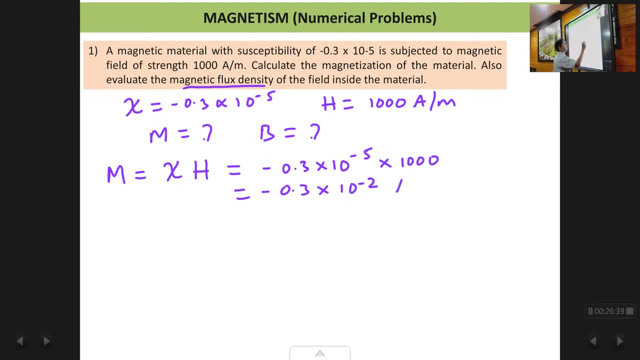 H has units of ampere per meter, so magnetization also will have units of ampere per meter. so this is the first part of the problem. we have calculated the magnetization in the material. next part is to find the magnetic flux, density B, and what is the formula of B?